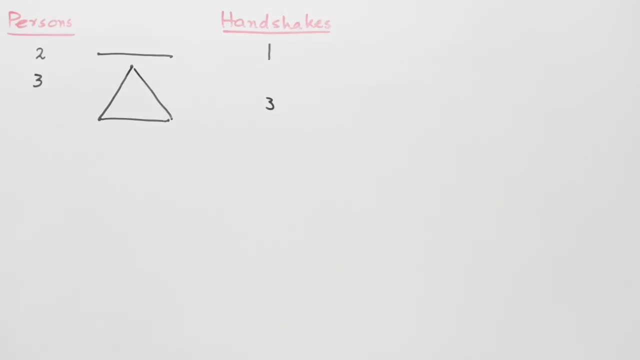 So there are three handshakes Now if we have four persons, so one, two, three, four, five, six. So there are six handshakes Now if we have five persons: one, two, three, four, five. 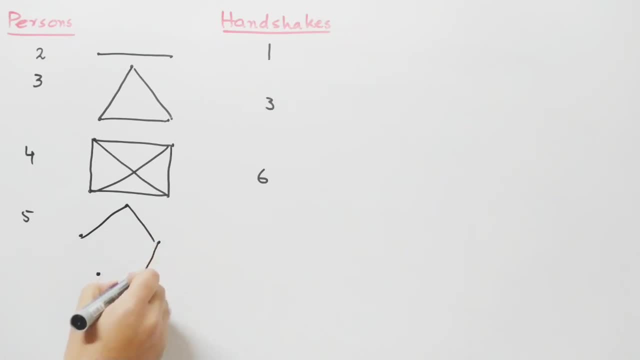 One, two, three, One, two, three, four, five, six, seven, eight, nine, ten. So there are ten handshakes. Now we can write: three is equal to two plus one, six is equal to three plus two plus one, and ten is equal to four plus three plus two plus one. 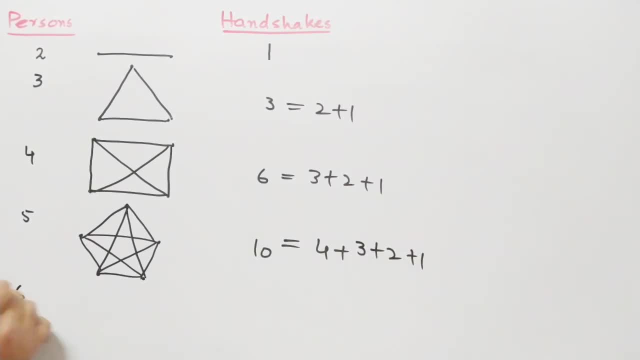 So look at the pattern. Now. if we have six persons, We can write five plus four plus three plus two plus one, following the same pattern, which is equal to fifteen. Now if we have n plus one persons, so the handshakes will be sum up to n. 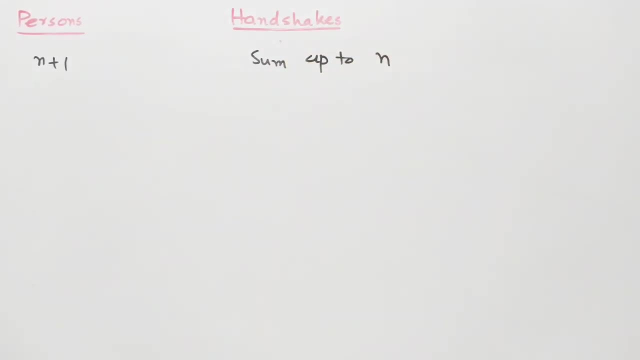 And we know that sum up to n is what It's. one plus two plus three up to n is equal to n. into n plus one divided by two is equal to this. So now, if we have seven persons, there will be how much handshakes. 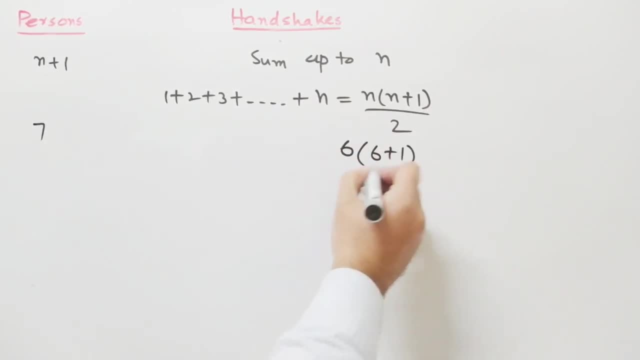 Just, we will use the formula Six into six plus one divided by two, And that will be equal to twenty-one. Now we are coming to our question. In our question we have sixty-six handshakes. So n into n plus one divided by two is equal to sixty-six. 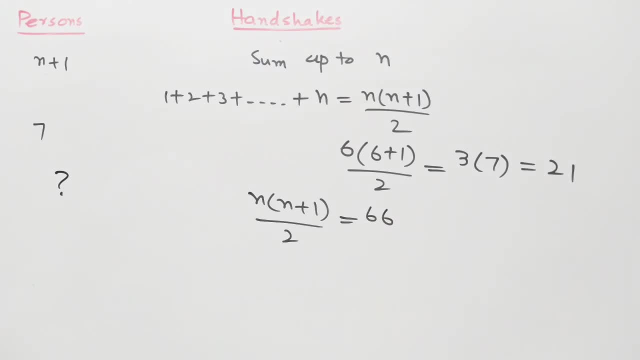 And we have to find the n. Then we can write n plus one. We can simplify this: n square plus n is equal to one thirty-two. Then we can write n square plus n minus one thirty-two, Which is a quadratic equation. 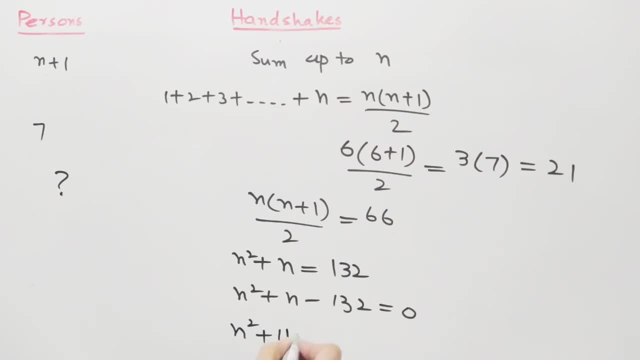 And then we can solve this quadratic equation by quadratic formula or by factorization. Suppose, by factorization we are writing n square plus twelve, n minus eleven, n minus one. thirty-two is equal to zero. Here we will take n common, So n into n plus twelve minus eleven. 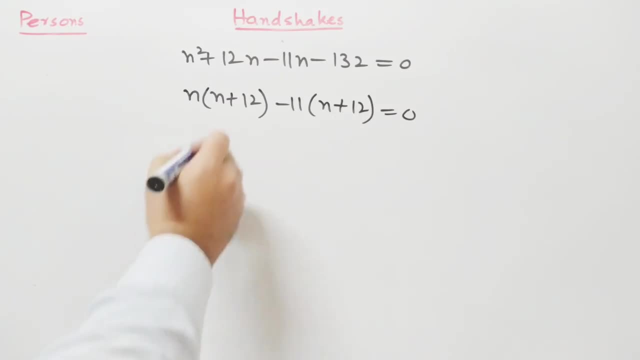 n into n plus twelve is equal to zero. n plus twelve into n minus eleven is equal to zero. n is equal to minus twelve or n is equal to eleven. So we are finding the number of persons, So n is equal to eleven. 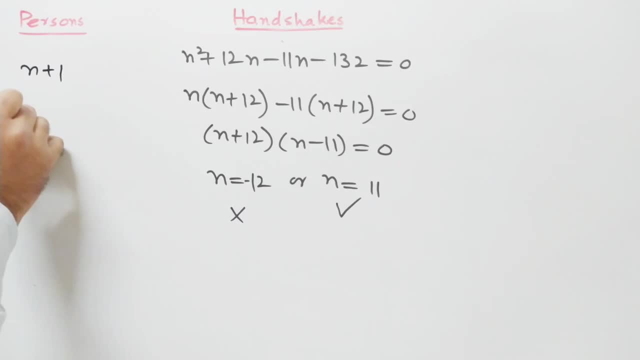 And we cancel the negative. So n plus one persons. So eleven plus one is equal to twelve. So the answer for this Question is twelve. So if we have twelve persons, there will be sixty-six handshakes. 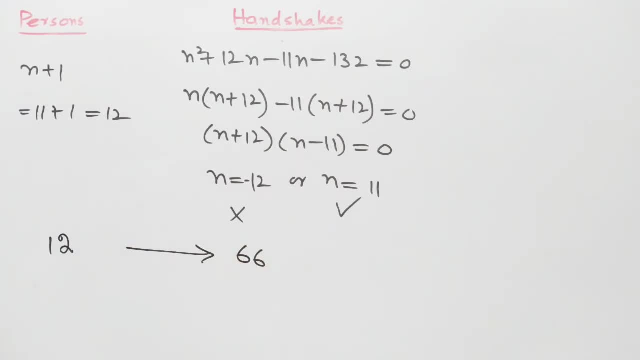 Twelve persons, So sixty-six handshakes. So now we can solve any question like this: If we have given the number of persons, so we can find handshakes, And if there are handshakes we can find number of persons. 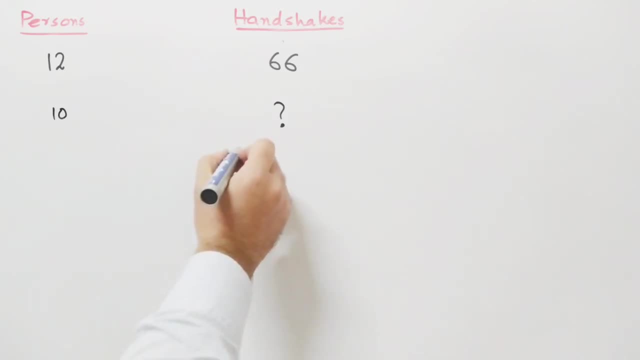 Suppose we have ten persons In this. look at this example: If we have ten persons, there will be how much handshakes you just put in And n is nine because we are writing, ten is n plus one, So and this is equal to forty-five. 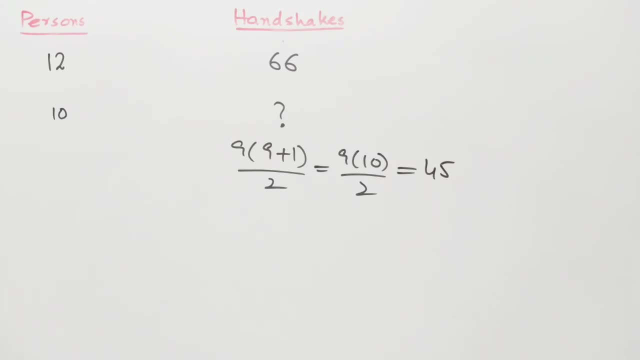 So if we have ten persons, there will be forty-five handshakes. Now, if we have forty-five handshakes, we have to find ten persons. So we will write n into n plus one divided by two. Is it clear? 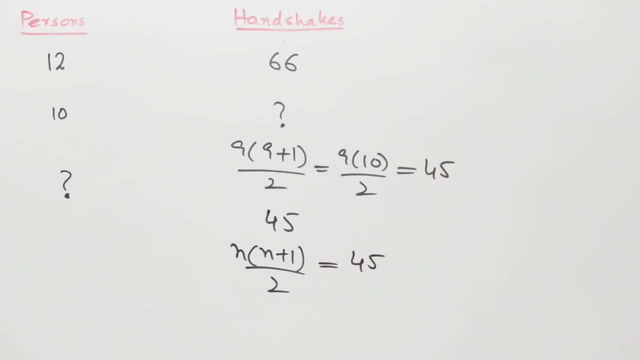 So n is equal to forty-five And we can write it: n square plus n is equal to ninety, And n square plus n minus ninety is equal to zero, which is again a quadratic equation, And we can solve any quadratic equation by factorization or by quadratic formula.